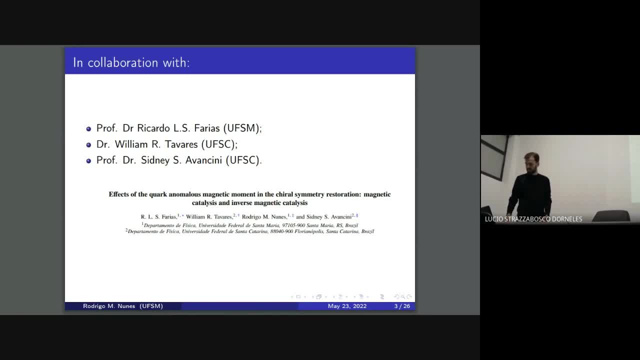 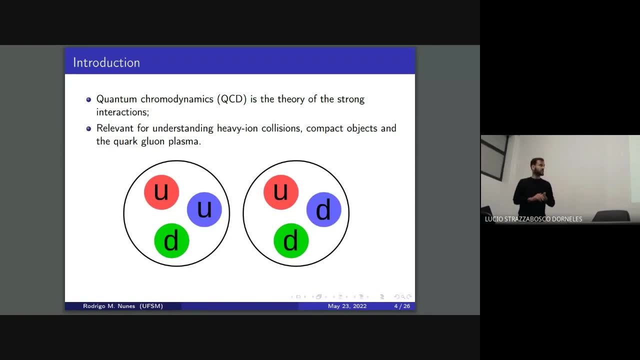 William Tavares and Signe Albansini. So let's talk a little bit about QCD first. So the QCD- quantum chromodynamics- is the theory of the strong interactions that detects the dynamics between quarks and moons. The study of QCD is relevant for many physical systems, such as heavy eye collisions. 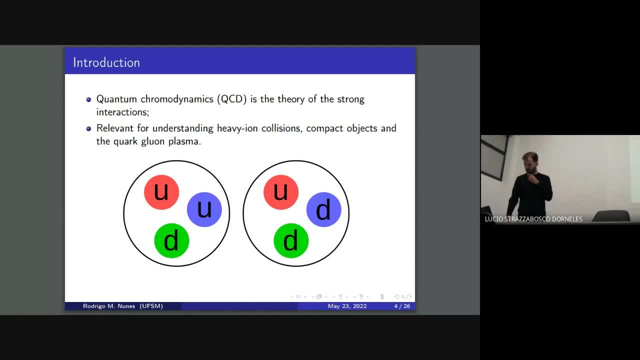 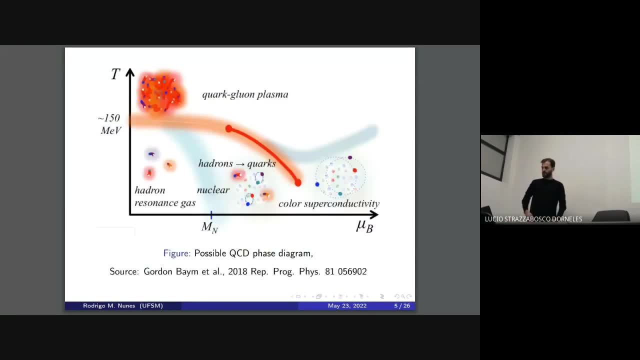 compact objects and quark-gloom plasma. Here we have a phase diagram, a possible phase diagram of QCD. In the vertical axis we have the temperature and the horizontal axis the chemical potential. So at low energies, that is, low temperature, low chemical potentials. 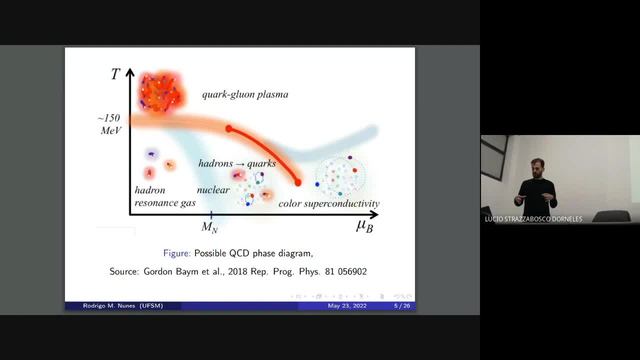 QCD has a property called confinement, where the quarks are confined within the hydrons. But for higher energies the QCD matter turns into what we call the quark-gloom plasma, where we have three parts. It happens both for higher temperature and higher chemical potential. 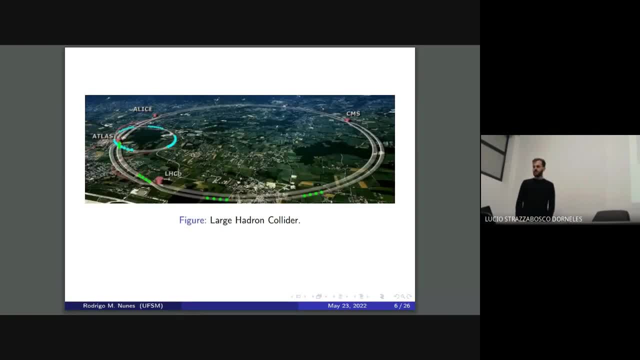 So one of the main objects of study of QCD are heavy iron collisions due to the higher energies And in the last phase diagram we just took some visiting of QCDes driving quarks, and quarks where theoys, quarks where weight. that is the difference between the azimuthic tomarcation. 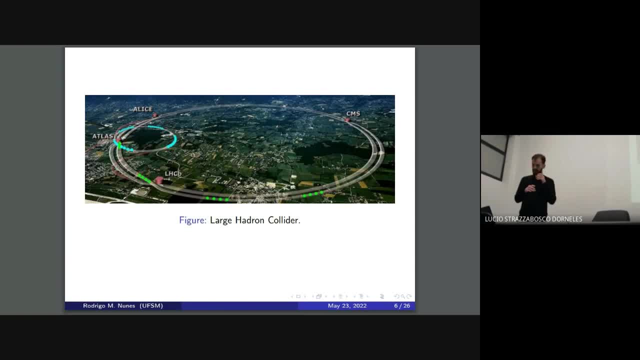 for high energy verdiases and the quarks where the elevating hegemonic durations is. so deaths and movement over servants of quarks In the This particular case of QCD in the image in the uwagę to the left you can see that QCD lambda is populated between Donna vähän. 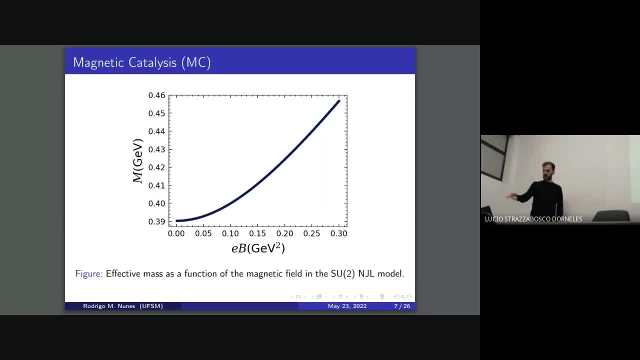 Zapadi and the calcr in the arc서�aver difficulinet characterized for the increasing of the chiral condensate as the magnetic field increases. In the NGL model, for example, we can see this as the increase of the mass. 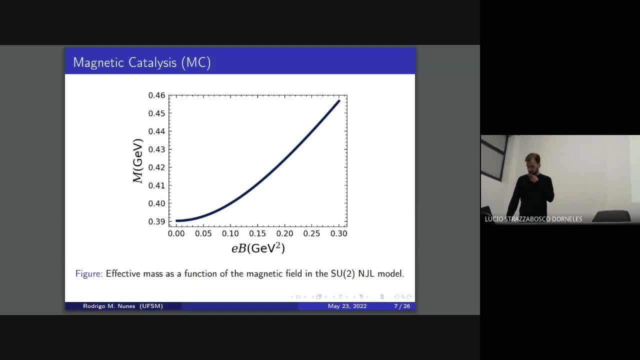 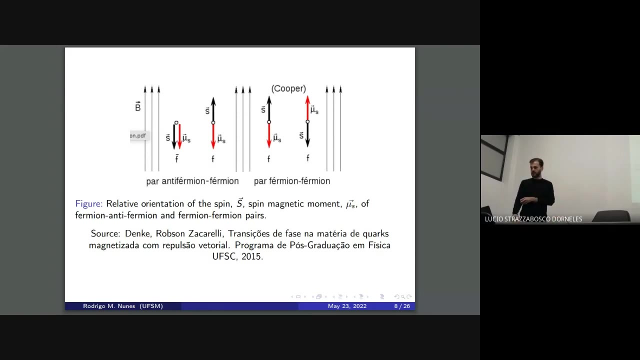 as a function of the magnetic field. This effect is not exclusive for quark matter, but for fermions in general. An oversimplified way to understand this is looking at the relative orientation of the spin and the magnetic moment of spin of a fermion-antifermion bell. 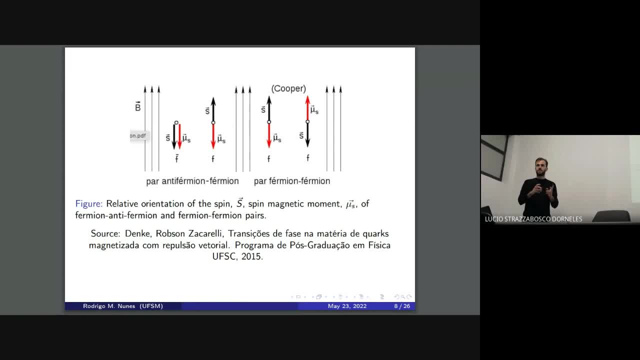 For example, the negative charged particle, the spin in the magnetic moment will be always pointing in the same direction, And for a positive charged fermion the direction will be opposite. So when we have a magnetic field, this magnetic field will be. the particles will align with the magnetic field in the same way. 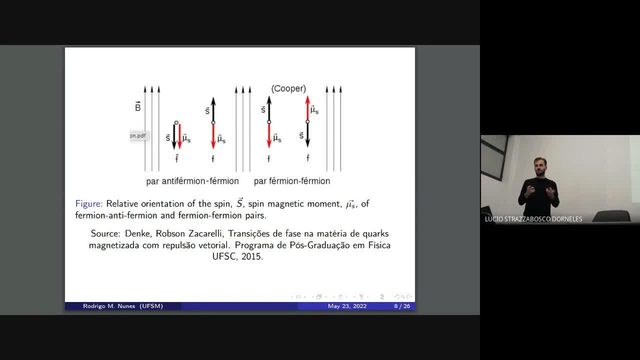 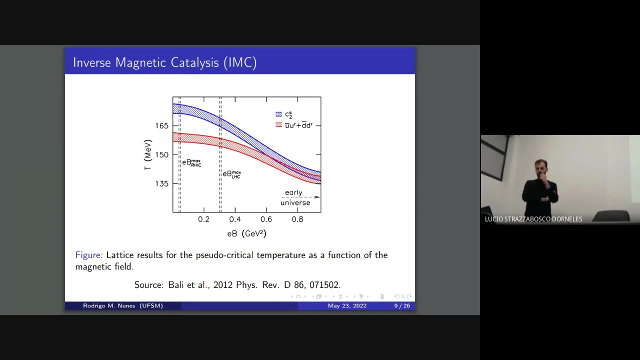 so the condensate will be strengthened. The opposite behavior would be observed for the fermion-antifermion bell, where the magnetic field tells the chiral part Well, effective models We have. basically have many ways of studying KCD, but one of the main 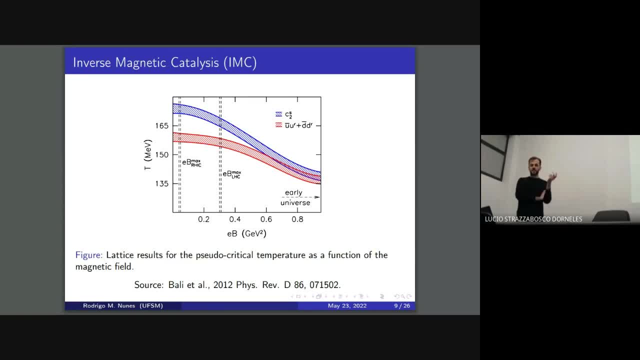 ways is through Lattice simulations And another one is through effective models. So Lattice simulations will give us rate results for lower chemical potentials, who are very high. So Lattice simulations will give us rate results for lower chemical potentials, who are very high. 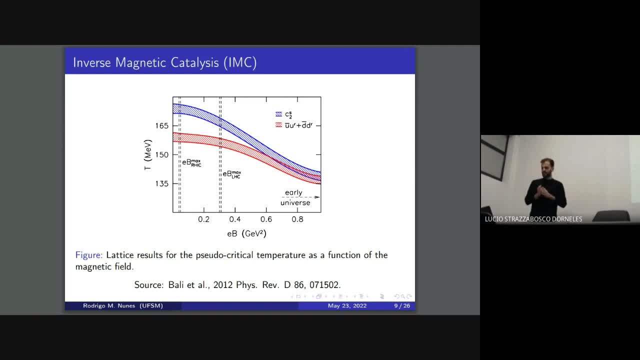 For higher chemical potentials. there's this time problem, so we need effective models. There's a contradiction between effective models and Lattice simulation. Effective models predict that magnetic catalysts should happen for every temperature, but that's not the case when we look at Lattice simulations. Lattice simulations: they confirm magnetic catalysts. 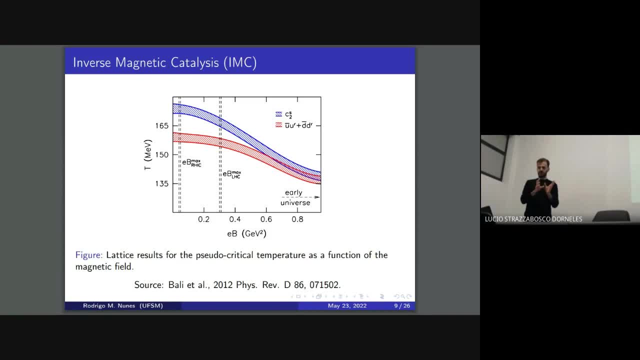 for low temperatures. but we see the opposite happen when we have temperatures close to the pseudo-critical temperature, where the magnetic fields start acting as a catalysis to the restoration of the symmetry instead of breaking the symmetry. We call this the inverse magnetic. 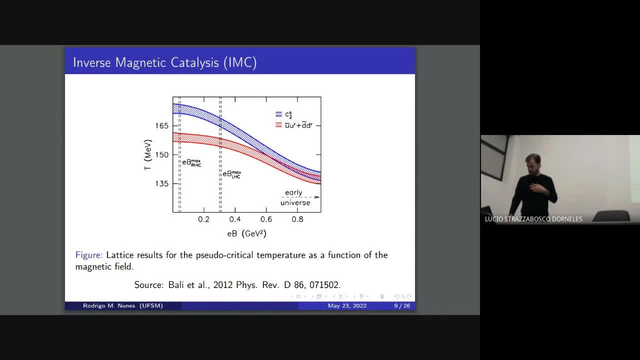 catalysis. We can see this for the…. We can see here the pseudo-critical temperature. We can see here the pseudo-critical temperature. It's the temperature for the restoration of the symmetry. It will decrease as the magnetic field increases. So in order to explain the contradiction, there's several attempts been made. One of them is the: 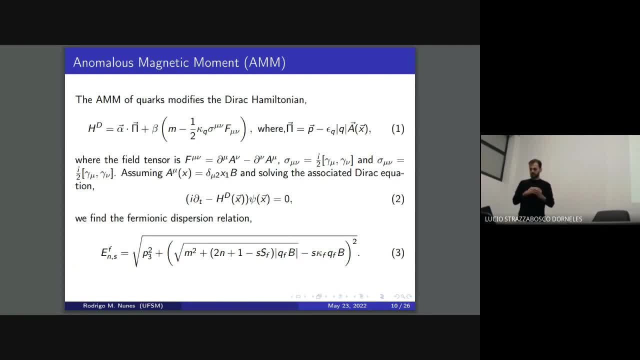 inclusion of the anomalous magnetic moment of Quarks. The… of the AMM of Quarks. So the AMM of Quarks will modify the direct Hamiltonian by the… for using this…. this term here will modify the direct Hamiltonian. It's an additional term. 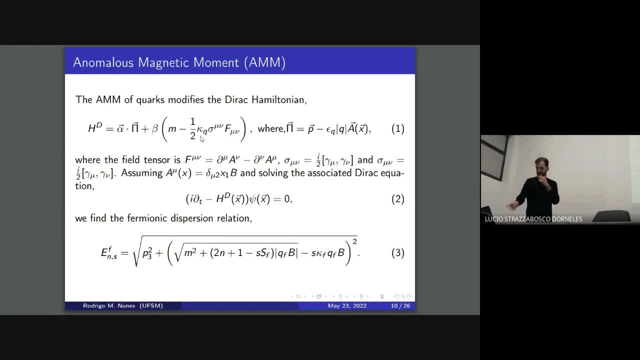 By this term here It's an additional term that… comes for the inclusion… from the inclusion of the AMM, And when we solve the associated Dirac equation, we can find a dispersion relation given by equation three, whereas this… this negative term here will be a minus contribution to the effective mass. 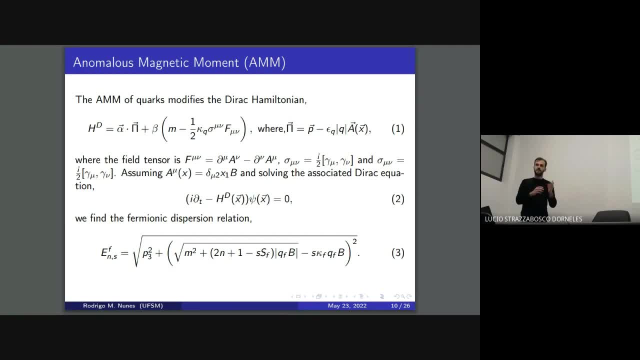 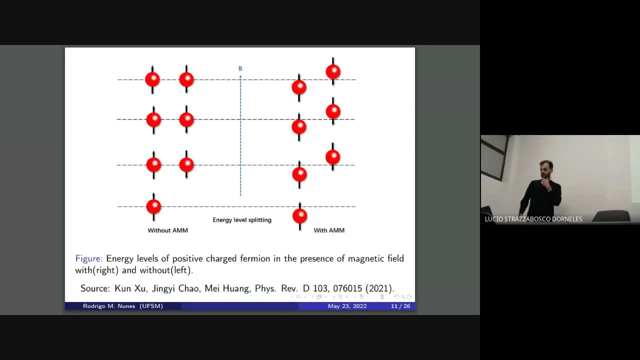 So we believe that it could possibly explain the inverse magnetic catalysis. If we look at the energy levels, when we consider the… the effect of the AMM, we see a sort of a Zeeman splitting happens, sort of similar to that that could help carry… that will change the. 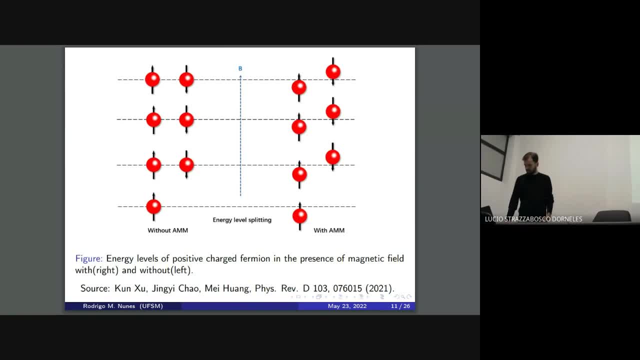 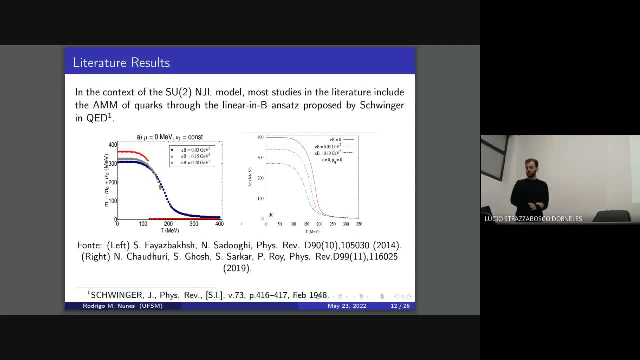 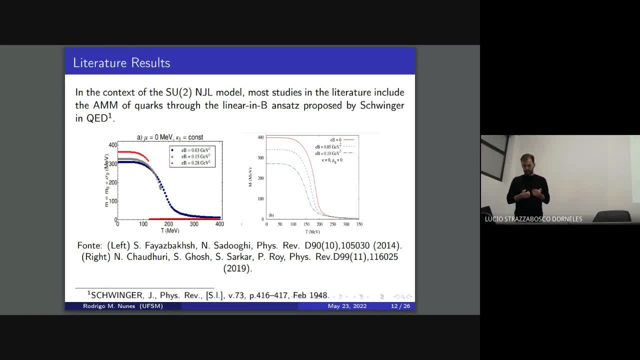 It's the term that I've shown before, But in general, most results in the lecture here are completely different. For example, here we have two results where the same calculation was done. The only thing that…. Two minutes, all right. the only thing that changes the is the regularization procedure. as you can see, here we 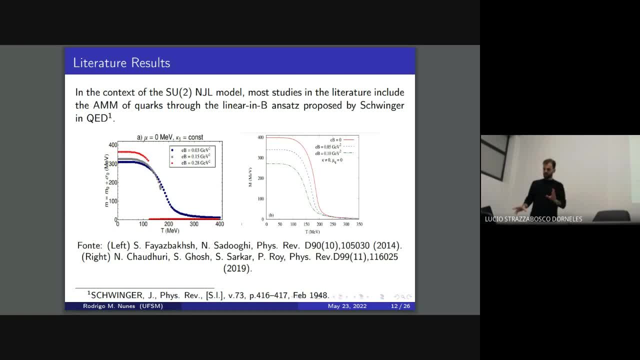 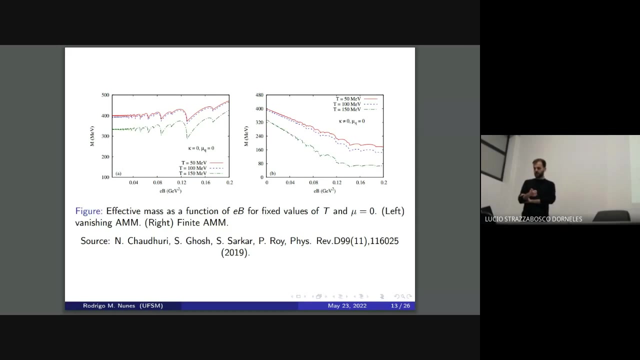 have a magnetic catalysis happen on the left panel for low temperatures and then we have stuff similar to a first order phase transition, but in the right panel we have inverse magnetic catalysis happen everywhere and the restoration of course has a smooth crossover. not just that, but we also see in most of the uh this studies and physical oscillations. 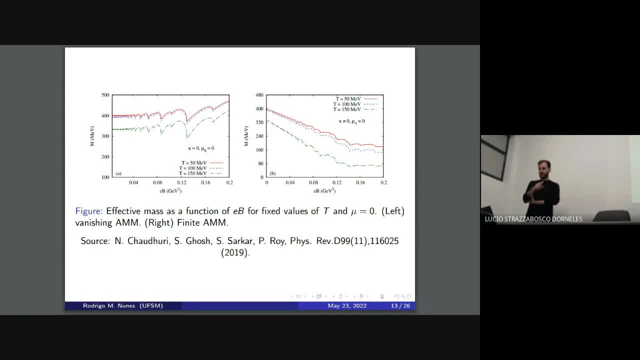 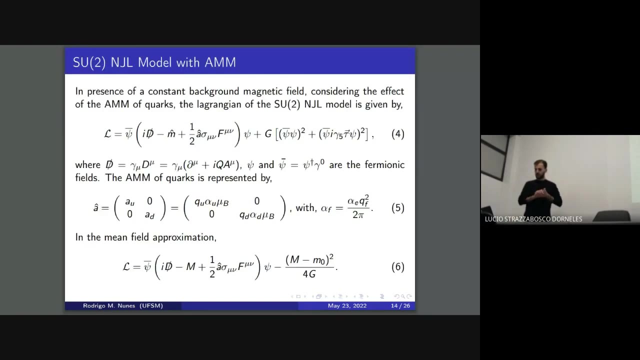 happen in the mass as a function of the magnetic field, something that shouldn't be happening usually, especially not when you have zero chemical potential. so the njl model, for with two flavors, we're going to consider the amm of parts. the lagrangian will be given by 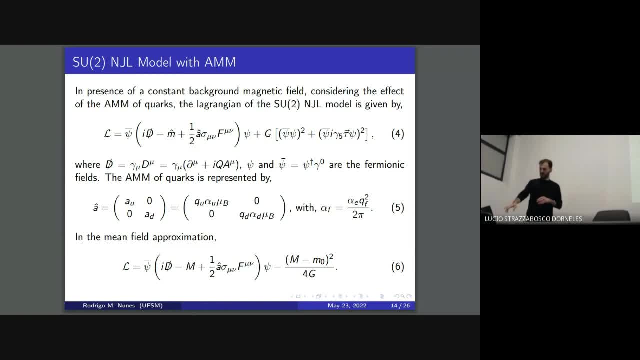 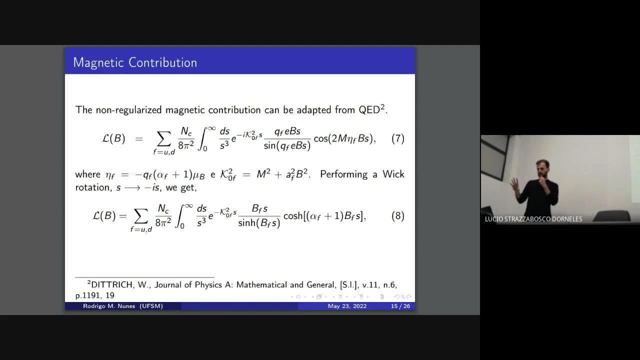 cogent four, where the a hat represents the amm, the effect of the amm in the mean field of impersonation. we have equation six, the lagrangian into impersonations, we will adapt the magnetic contribution from qed. we can do that because the equation that we have to solve is basically the same. we just need to adapt the qed constant for 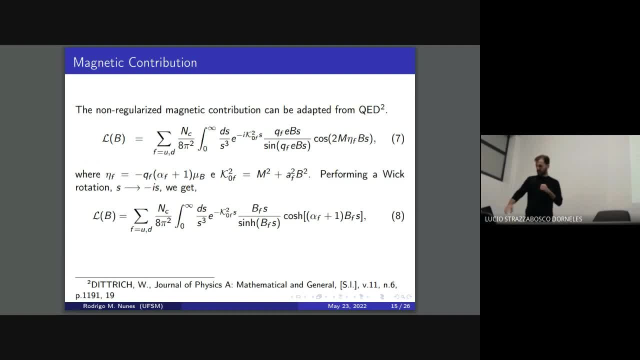 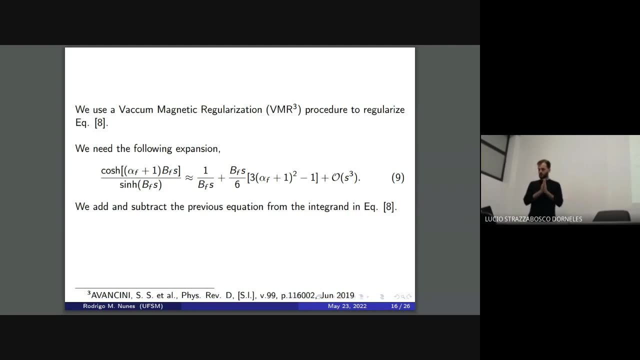 qcd constants. and if we do a weak quotation in equation seven, we get occasion eight. the equation makes divergence, so we need to implement a regularization procedure. we choose a vacuum magnetic globalization. to do that we just need to expand the term cosine by sine, uh, hyperbolic cosine by hyperbolic sine, and we get equation nine. 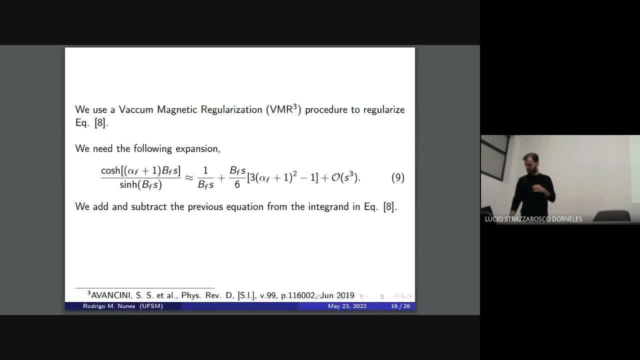 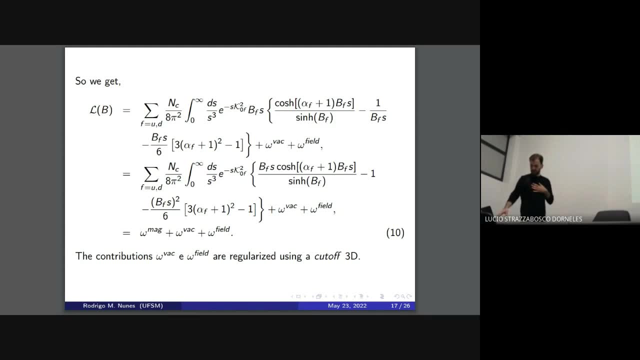 then we just add and subtract from the integral in equation eight, so we can get equation 10, where we have, when we have a pure magnetic contribution, that that's no longer divergent, we can integrate from zero to infinity with no problem, and we have omega vac and omega sinvac. 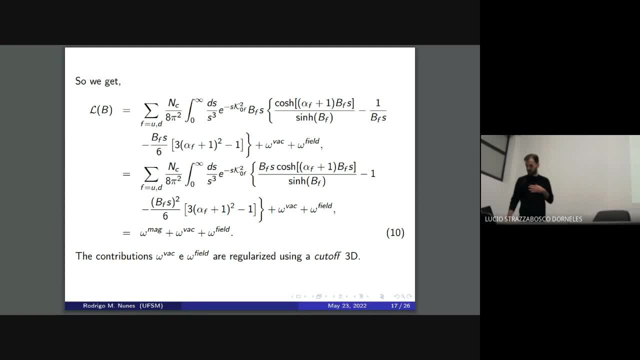 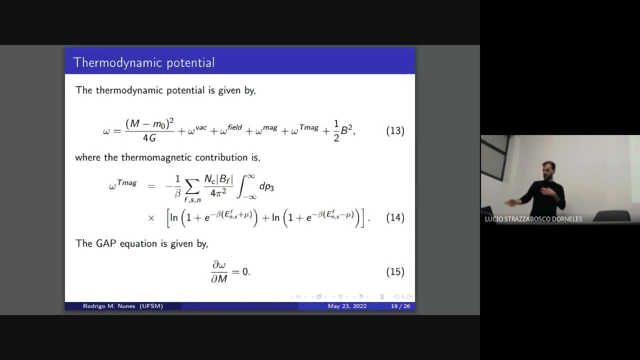 field, We need to use Akutov 3D to regularize it. Using Akutov 3D you get equation 11 and 12.. So the terminal and potential will be given by equation 13,, where the thermo-magnetic integration is given by equation 14, is the standard. 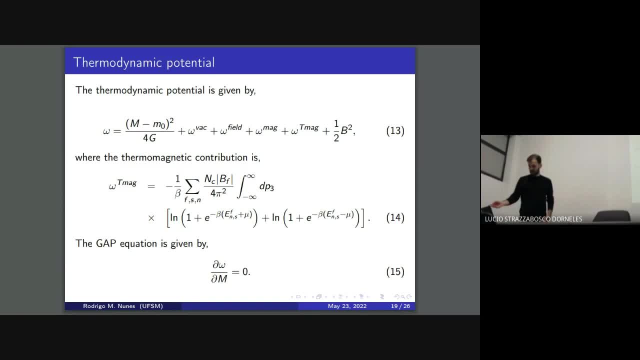 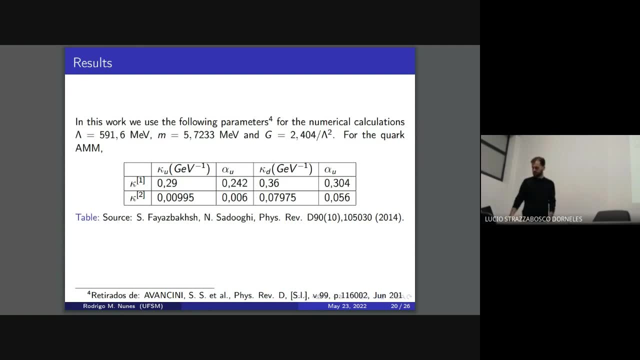 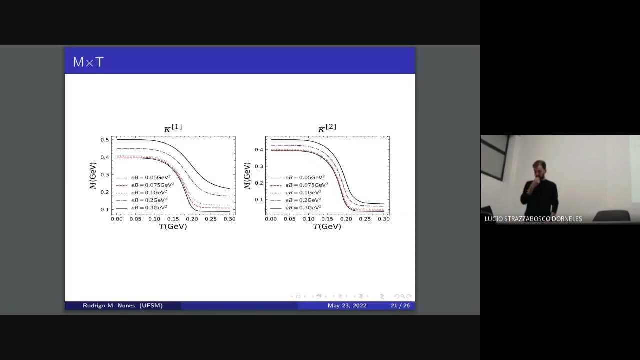 And the application of the equation. so we use the application of the term, the mass given by equation 15.. So these are the parameters that we use for the numerical calculations. Here we have the mass as a function of the temperature for two sets of: 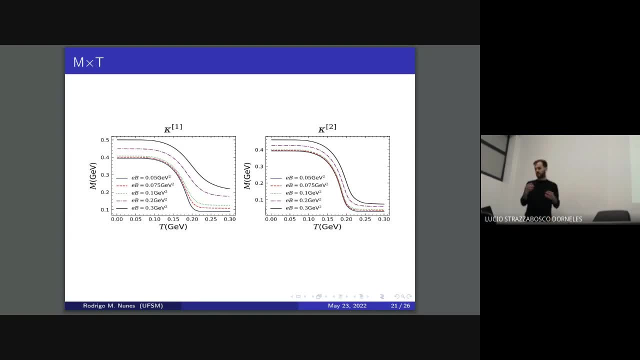 amm. The kappa one is a more sizable set and kappa two is the smallest values of amm. We can see that for low temperatures this magnetic catalysis is happening. We then the acceleration report as smooth crossover in both cases. To find the pseudo-critical temperature we just need. 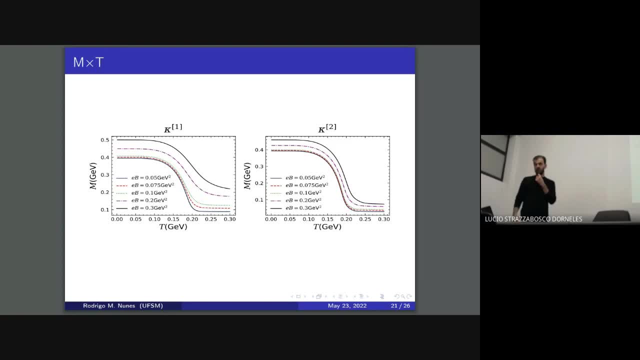 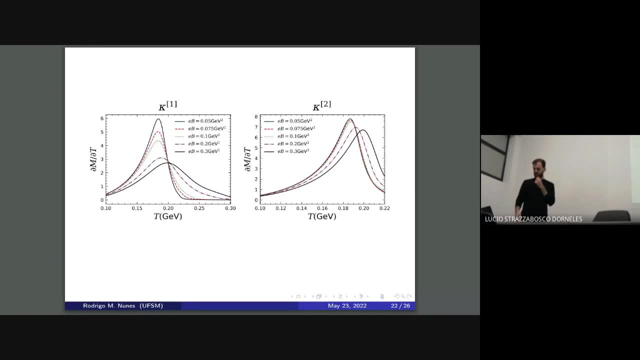 to determine the inflection points on those curves. To do that, we just calculate the derivative of the mass with respect to the temperature and the maximum that presents the pseudo-critical temperature. As you can see here: for kappa two, it's always increasing. kappa one: it's decreased just for a small window and then starts to increase again. 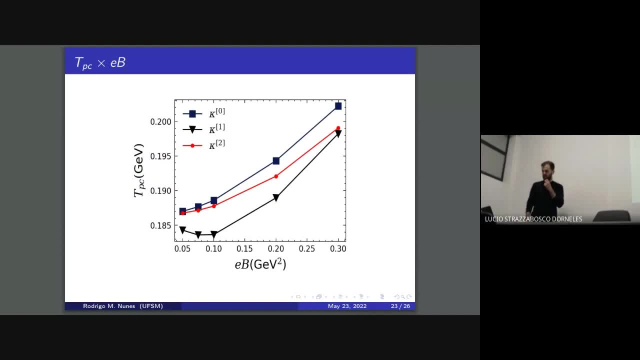 You can see this better in the pseudo-critical temperature as a function of the magnetic field. The blue line represents the case with vanishing and amm. As you can see here, there's a small window of inverse magnetic catalysis for this set, kappa one. 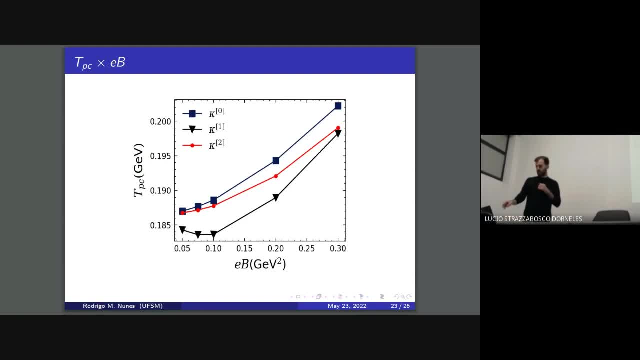 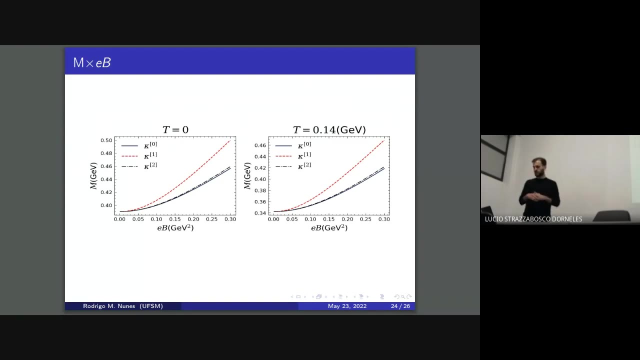 and the pseudo-critical temperature. it's always smaller than the case of vanishing. The blue line represents the case with vanishing and amm. Here we have the mass as a function of the magnetic field. As you can see, we no longer have physical oscillations happening. 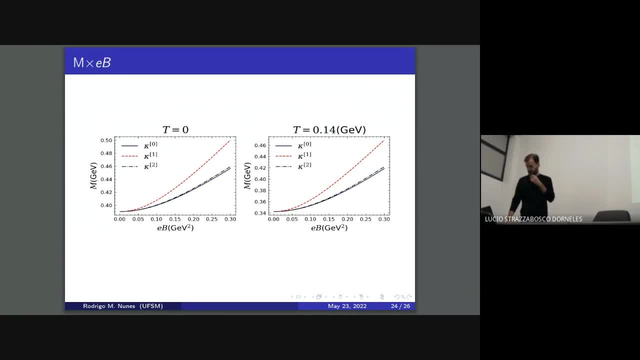 as expected for the VMR regularization scheme. In conclusion, the main effect of the AMM is in fact to reduce the critical temperature, but it only explains the inverse magnetic catalysis in a small window, As expected when we implement the VMR scheme for regularization.